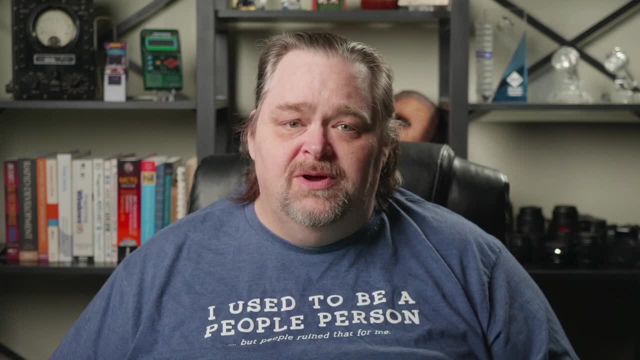 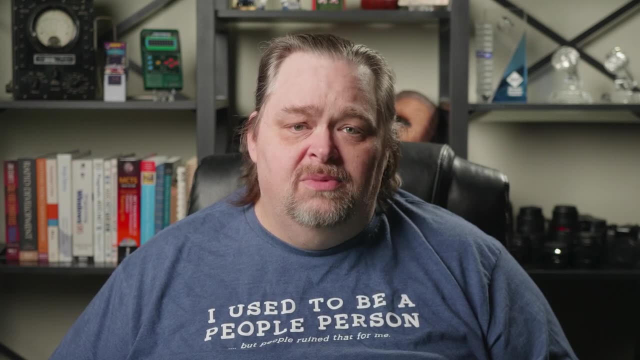 a user group. I want to be able to teach you something in your spare time. If this is your first time or you've been a long-time watcher without subscribing, please go ahead and hit the subscribe button and click the bell for alerts. It really, really does help. We've gone. 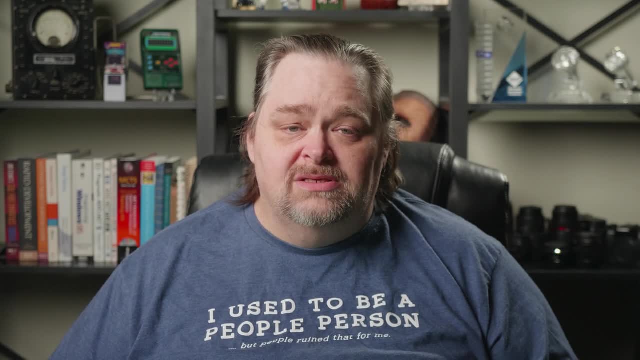 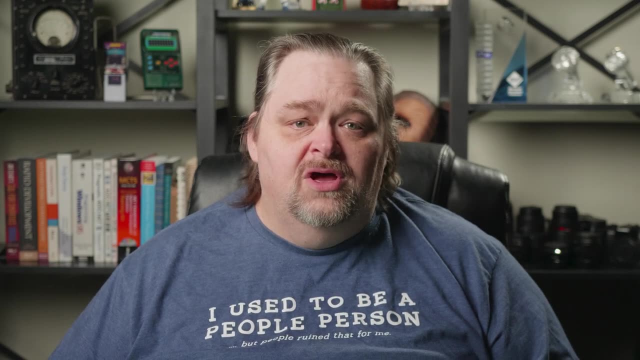 from just a couple of hundred followers to over 2,000 now. so I'm really excited, but the more the merrier. In this week's episode, I'm going to be talking about Vue 3.2's new feature of creating custom elements. This feature is going to allow you to package up a Vue component to be 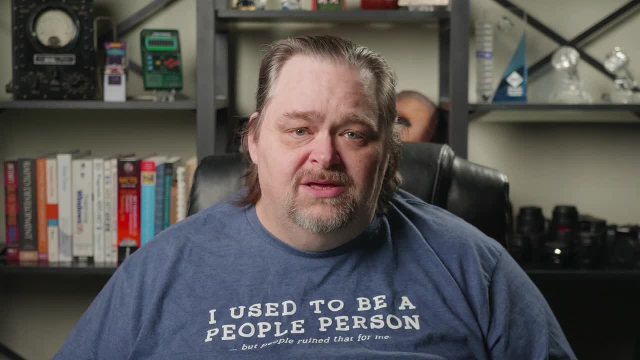 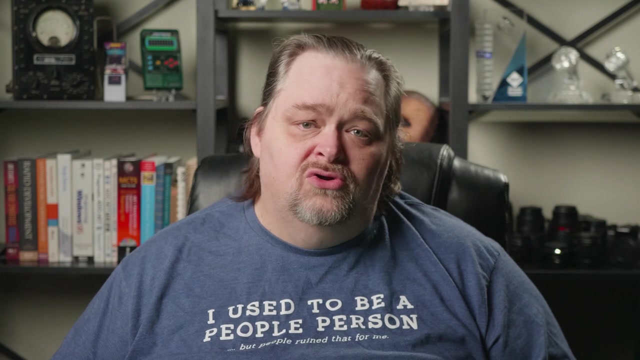 used directly on a website where you just have to include the JavaScript package and just use the custom element, And I can imagine some great use cases. We might want to create a reusable component that you use inside your CRM, or you want to package them up for end users to use without having to know or understand or know how to. 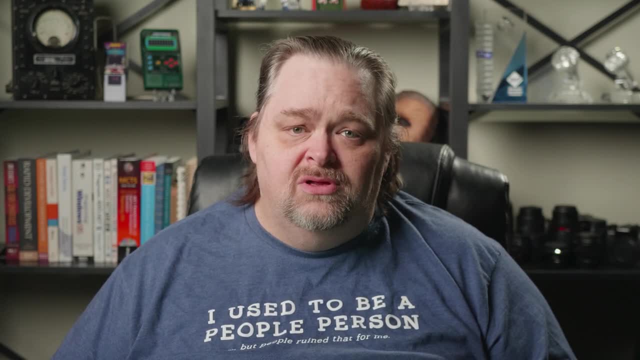 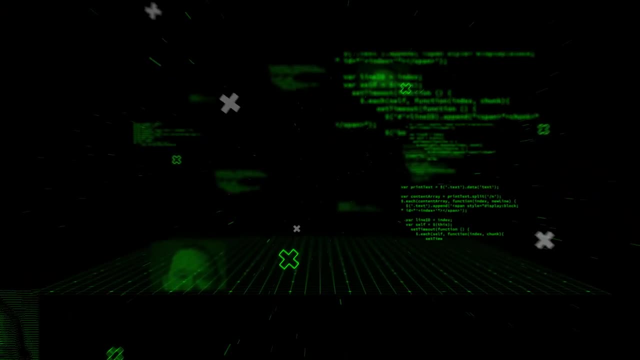 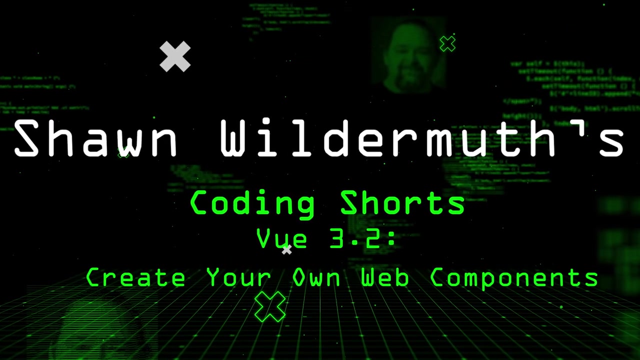 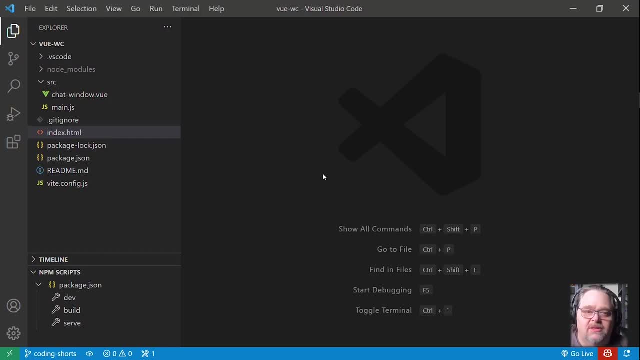 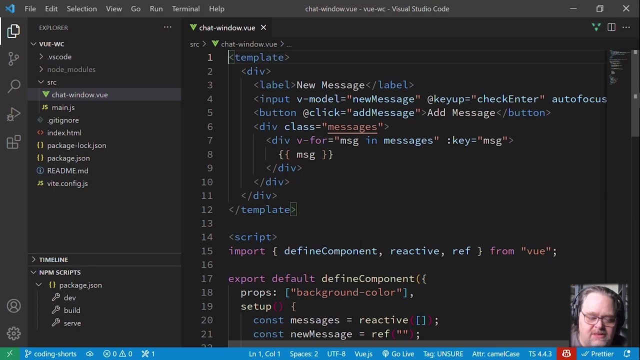 I want to show you a new feature of Vue 3.2 called Custom Elements. Let's take a look. So I have this beginning project and it's a simple app that has sort of a chat window, just a simple UI that allows someone to type a message in and it shows up in this message. It's 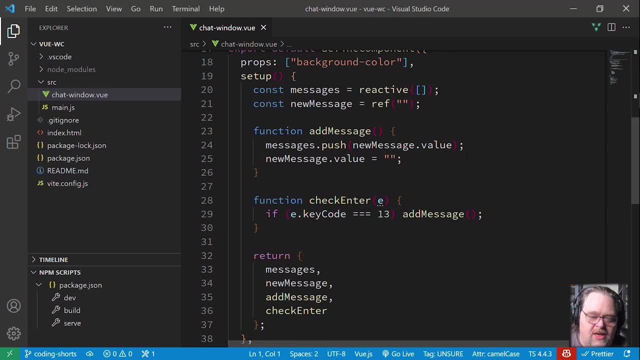 pretty simple: A couple pieces of state, the new message we're looking at and the message list, and then a couple of functions here to add the new message and clear the value, as well as to just check the status of the message. So I'm going to go ahead and do that. I'm going to go ahead and 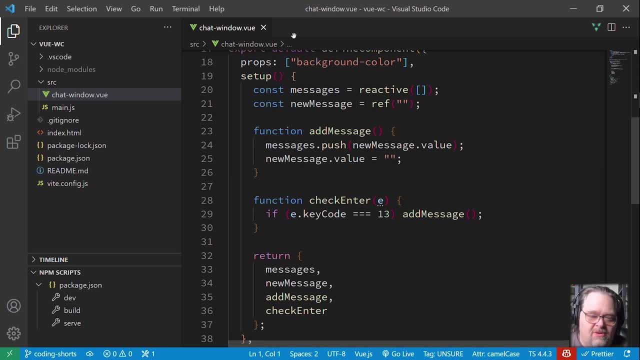 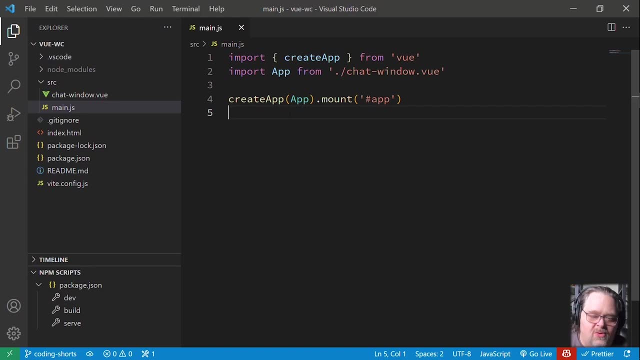 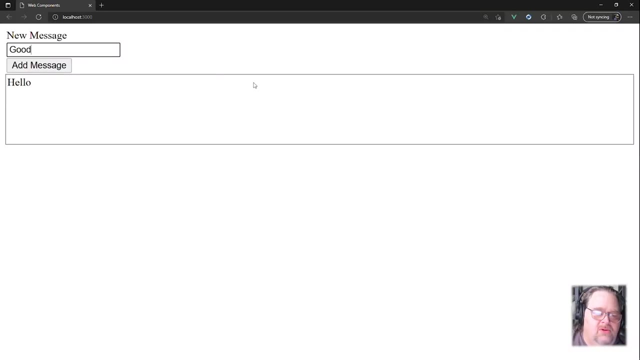 check to see if they hit enter and, if so, add the message. Not rocket science, a pretty simple component And like any simple Vue project, I'm just creating that chat window and then mounting it as an app And in the browser. it's pretty simple. So if I say hello, goodbye. 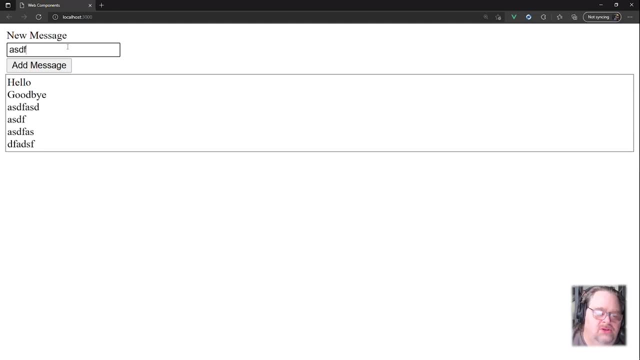 just shows it and would work, and it should grow as we go right. Nothing really amazing about this, but you can see it's sort of the start of something simple. So back in the code here I want to change this. I want to use custom elements instead. 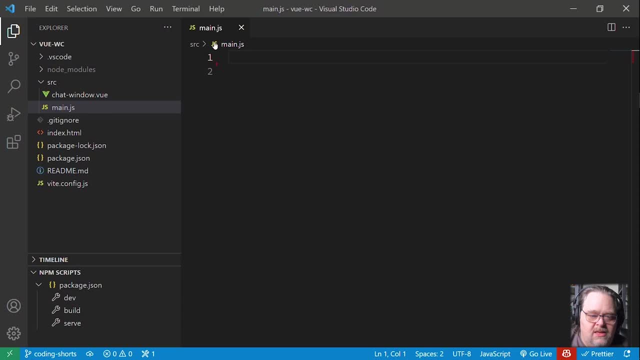 So let's erase this whole main and instead let's go ahead and erase the create app piece, and I'm going to actually rename this to chat, because what I want to do is I want to create an element by calling a Vue 3.2 feature called define custom element, And this is going to take our chat. 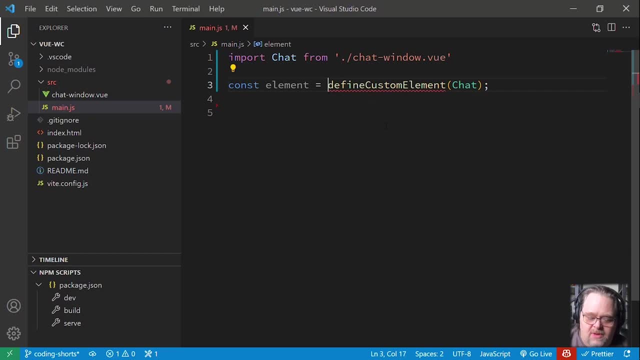 object and return this to the chat window. So I'm going to go ahead and do that, And then I'm going to create this custom element and let's see if we can just pull it out of Vue. Again, this is a Vue function And once we have that custom element, a wrapper around our component. 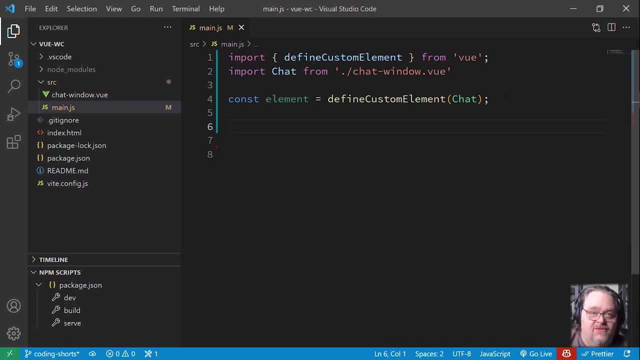 for something we can attach to the browser. we then have to go to the DOM and look at custom elements, and we need to define it. We're going to give it a name and I'm going to call it chat window. Now, this dash in the middle is important, and it's important because all 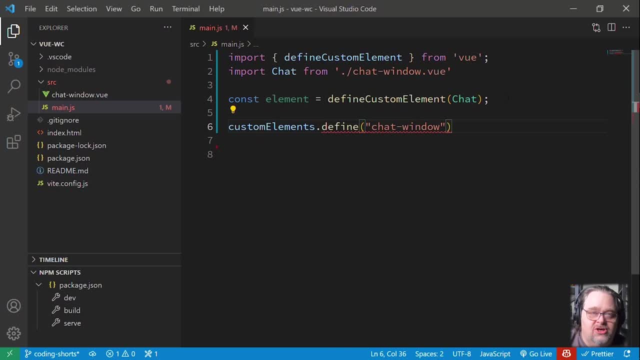 elements have to have a dash in them, And I think that's a security measure to make it clear that you don't have an element that is overriding a default element, the password input or something like that, And then here we're going to pass in our elements or telling the DOM: hey, if you see, 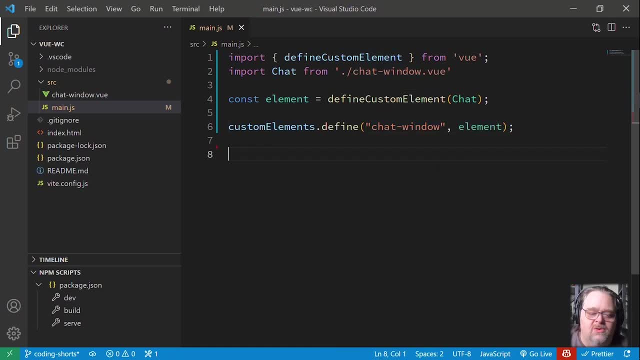 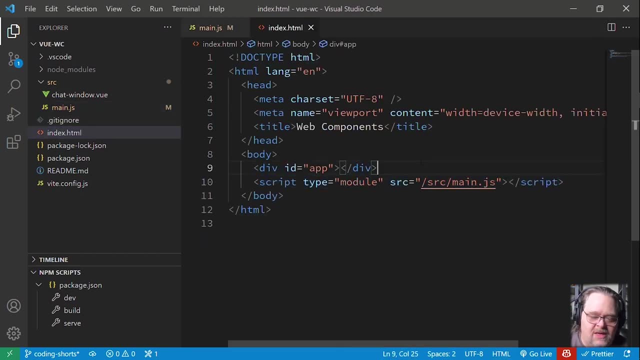 an object like this, use our wrapped element to actually run it So over in our HTML page. we're going to leave this. This is still going to load. Vite will actually still work with it. fine, But instead of having an app div, I'm going to do chat window. 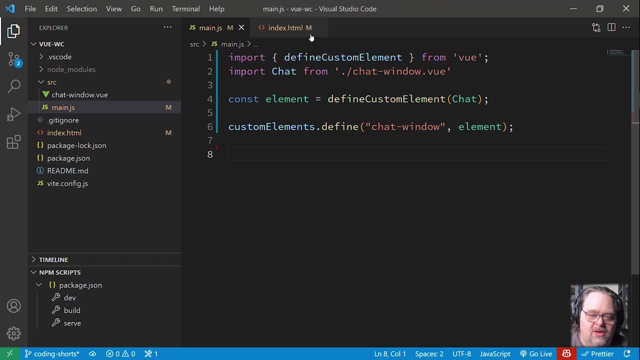 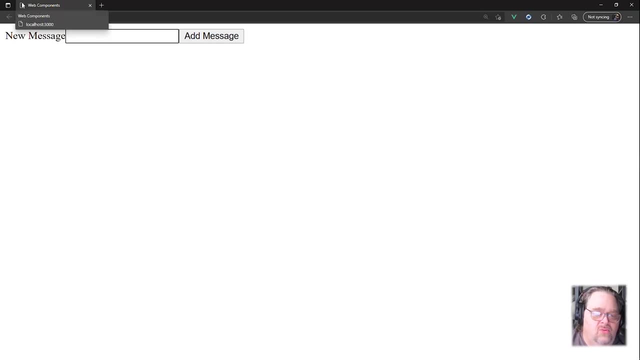 This is the name we gave it over here in main chat window. If we now go over, we can see that it worked. This is a functional web component. I can say hello, goodbye, And so we can use these on our page. but you might notice it looks a little weird. 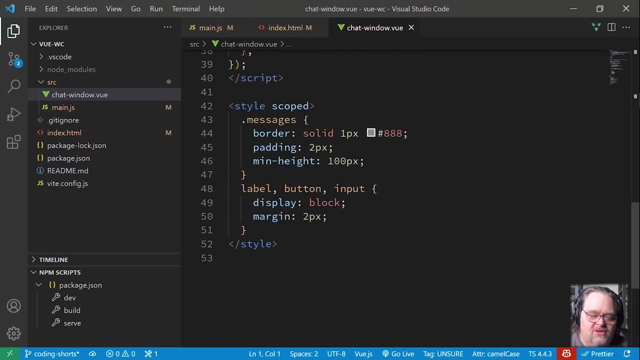 We look at the component again, You'll note that we have this style that we're going to call the CSS, And because components can't just reference or build the CSS, you have to have a way of taking these styles that are inside the component. This isn't necessary if 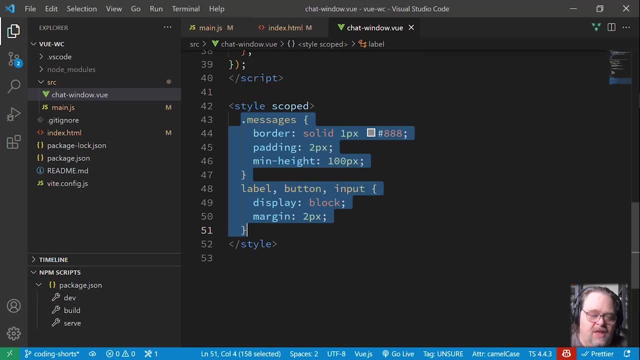 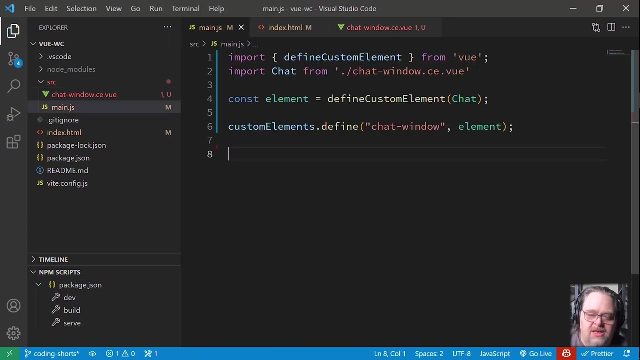 you don't want styles inside the component- if you just wanted them globally or something- And we need to stringify them so that they're emitted, And the short way to do that is actually to just call your file ce instead. This means a custom element, And let's make sure the main 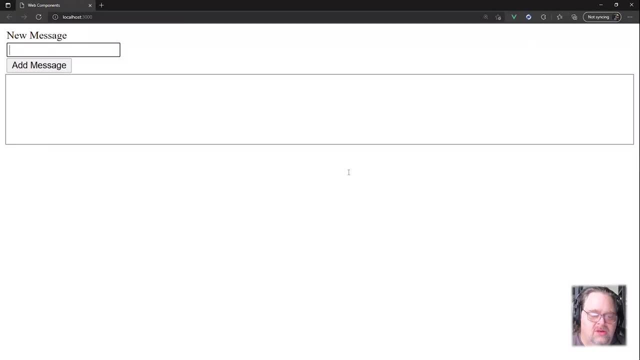 element is the name it did, And with that change we can see our styling came back, And so that was just a little change to allow us to do that Still works right the same way. Now you might think: why not just leave your spa as a mounted element? 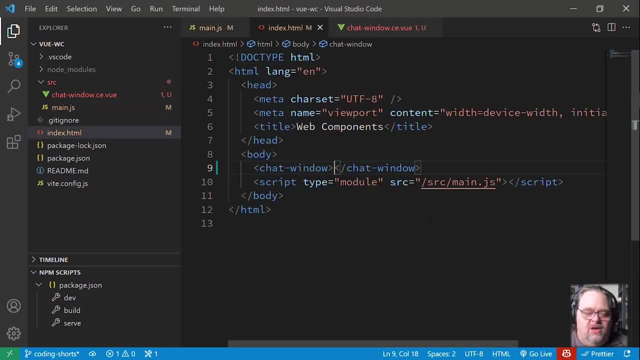 Well, that does make a lot of sense, But what we're really talking about is having the ability to have an element, maybe package this up as just a simple JavaScript, which I'm not going to get to show you in this coding short, But does work where someone could. 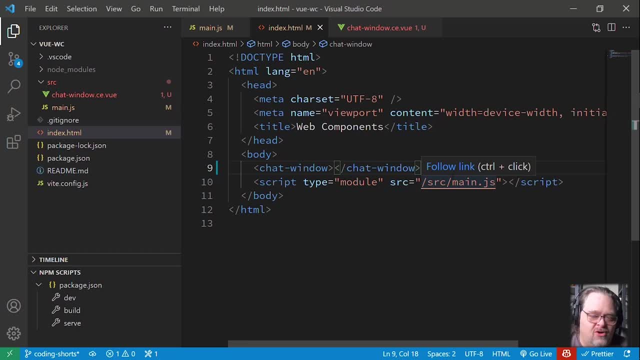 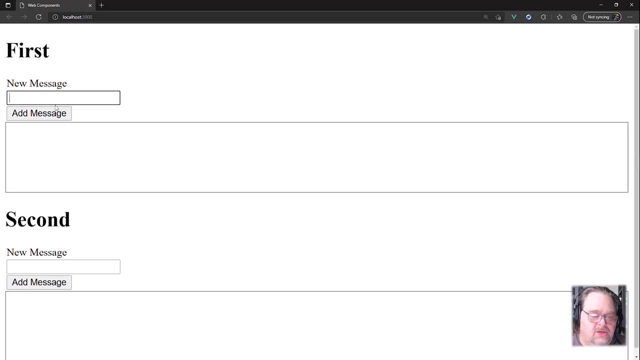 just bring in the JavaScript and then support these without having to think or know that they're ViewItAll. So let's take this, and I'm going to create a couple of copies of it to show that each instance of this is going to work on its own. Here we can see our first and our second. 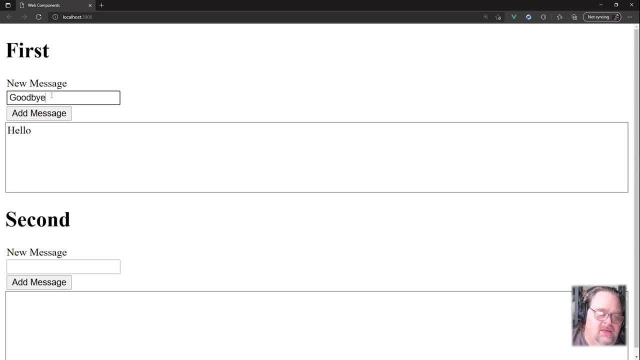 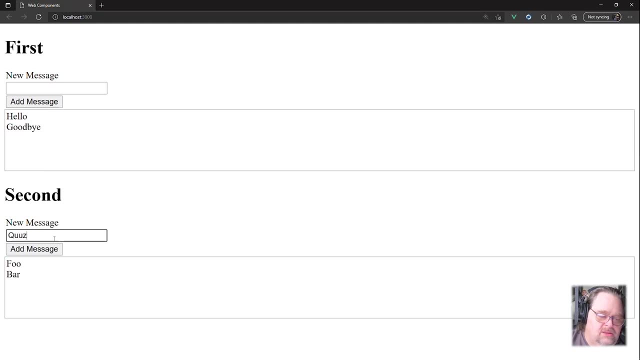 And if we say hello, goodbye, I don't know why I keep on wanting to type goodbye when I evidently cannot type it. and bar books: right, they're working independently, they're just their own instances of it, but in fact they aren't really. there's a single view runtime that's running both of them, which? 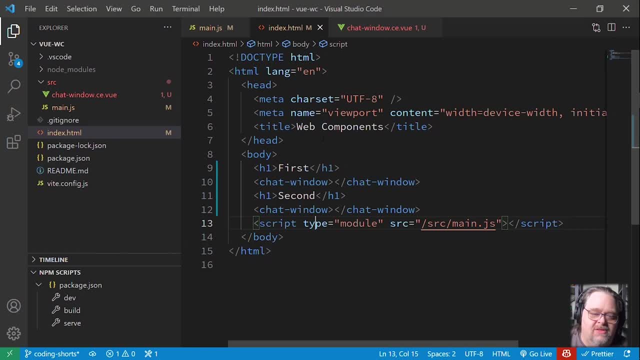 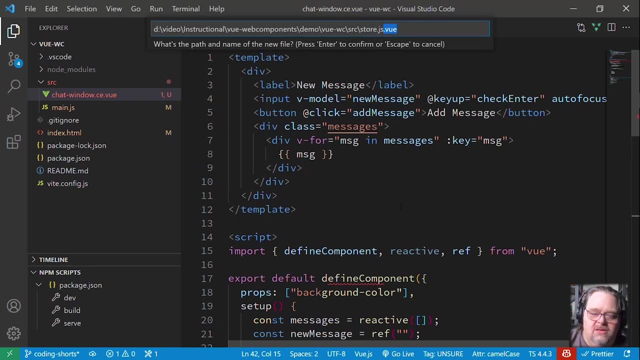 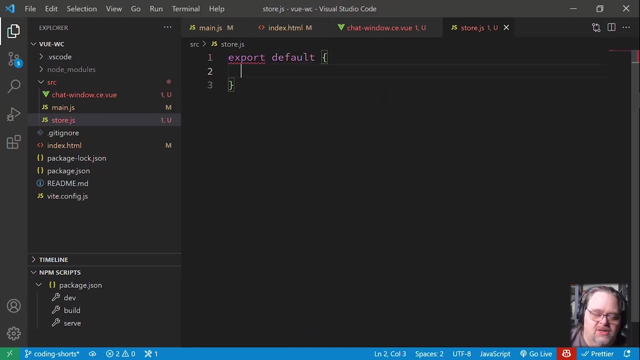 means that they could communicate between them. so how would we make that happen? let's come over to our chat window and let's create a new, let's say, storejs. now i'm not going to create a view x or anything, i'm just going to create a really, really simple store. so export default object and i'm 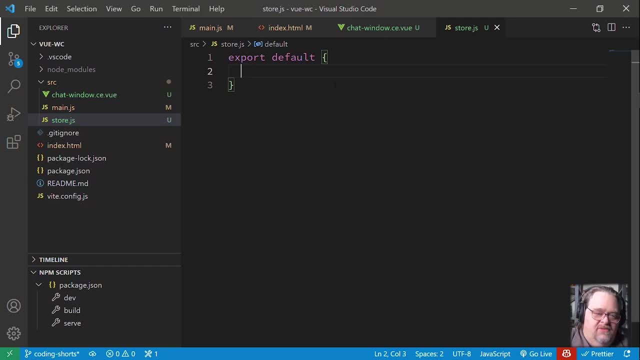 saying default object so that we get the same instance. right, if this were a factory, we wouldn't get the same instance and you can sort of control that. but this is a shared instance. anyone that imports this will get the same object back, and so i'll call this messages. i'll do what we did. 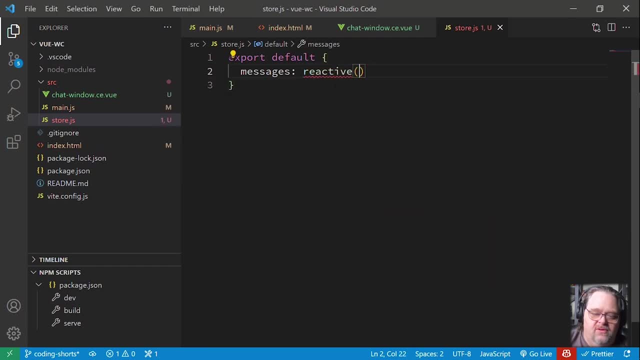 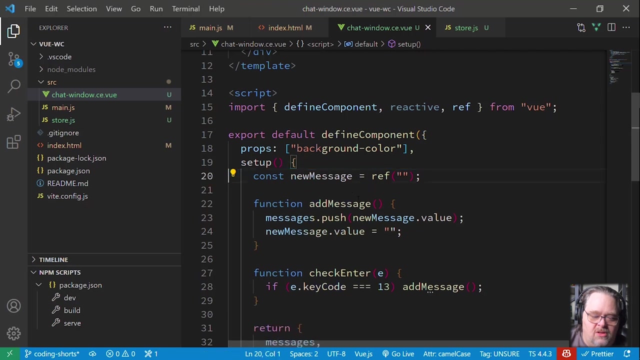 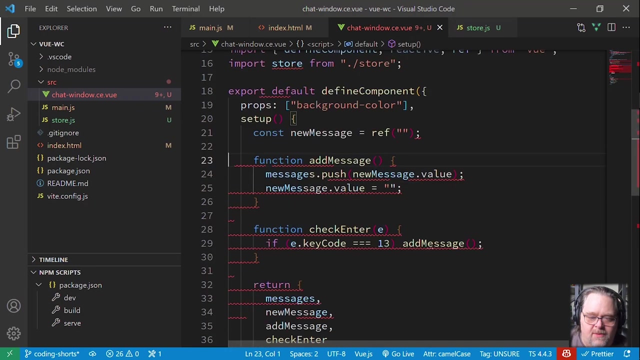 before, which is, put a reactive wrapper around an array and we'll need to bring in reactive, reactive and js. so that's our complicated store, but over in our component. let's take this messages and let's not use it at all. instead, we're going to import our store from store. we're getting a bunch of. 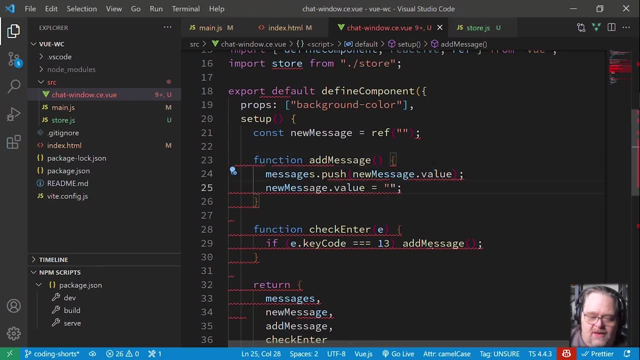 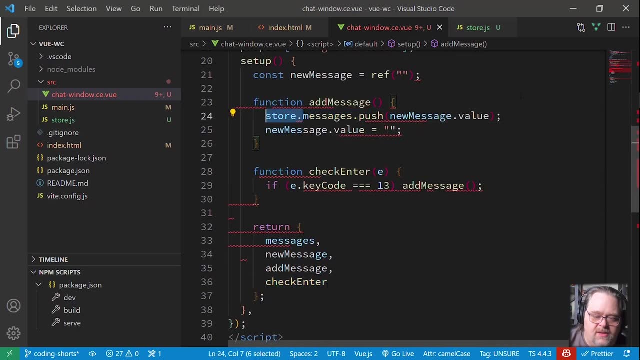 weirdness here. not sure why, but you gotta love the way this works. so in this case, messages doesn't exist, but storemessages- super does, and in that same way, our messages object here could just be storemessages, right? in this case we're talking about using a shared object and in an 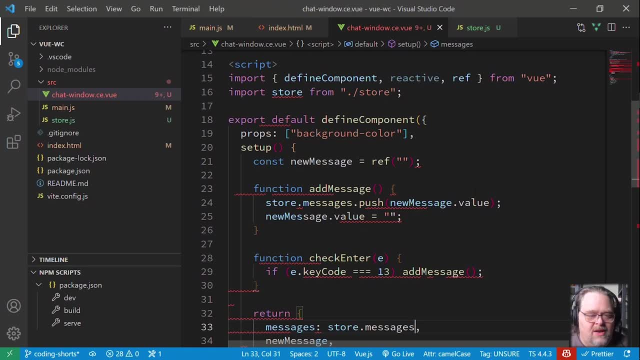 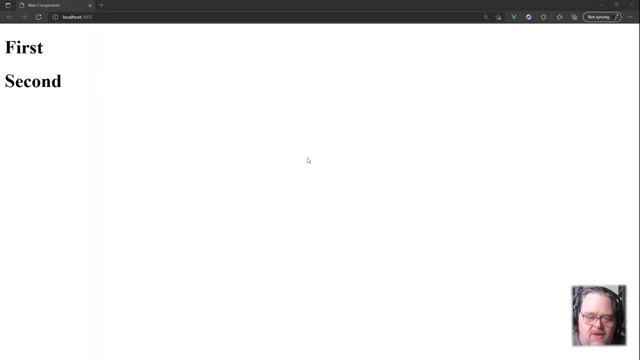 individual view instance. this would be easy, right? you would have a shared instance. you could share it between different components. that's great, but this extends to the way that this works. let's come back over here. we now have two, and when i say foo here you notice, because these are both. 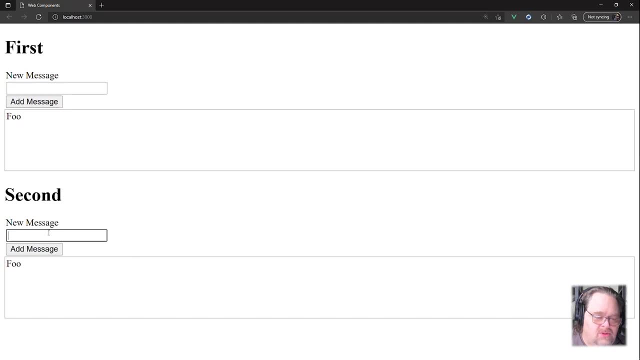 using that shared instance, we're getting the same object, so whether we add it in one or we added in another, they can actually get at these shared pieces of data because they're only using a single instance of you across them. there are some ways that you can defeat that, if that's. 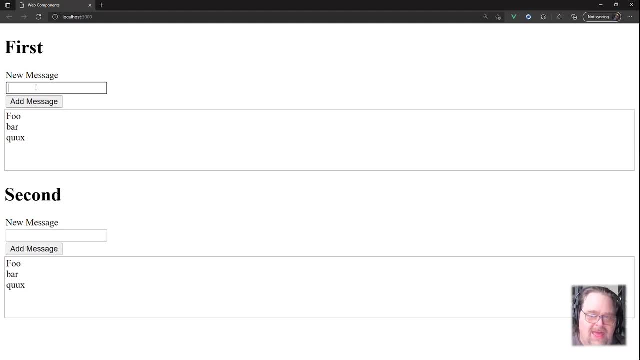 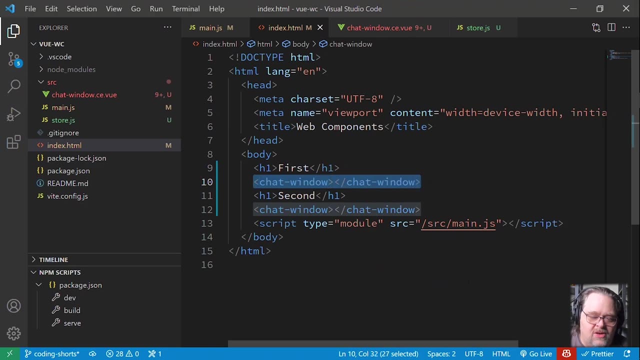 what you want, but this does allow you to have smaller components that might actually want to work together, and i like this, because the simplicity of using, you know, this idea of a chat window means that i could create something that might be useful in a cms and then have a. 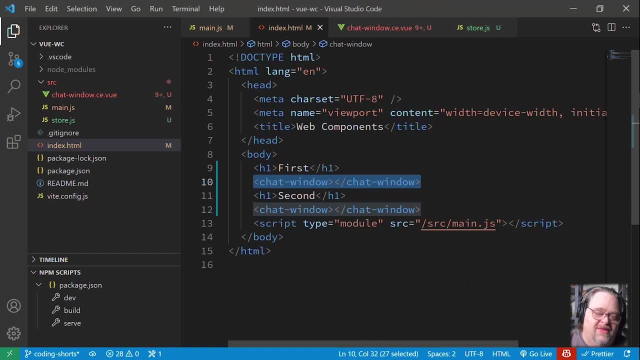 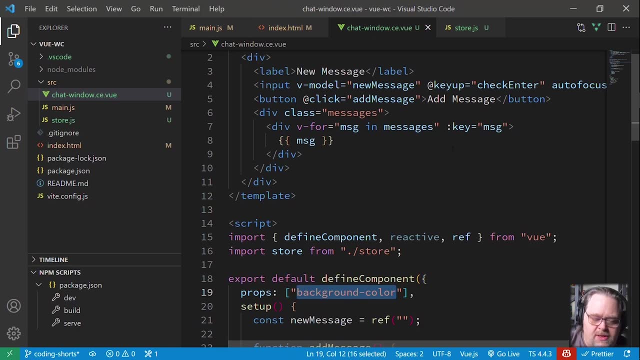 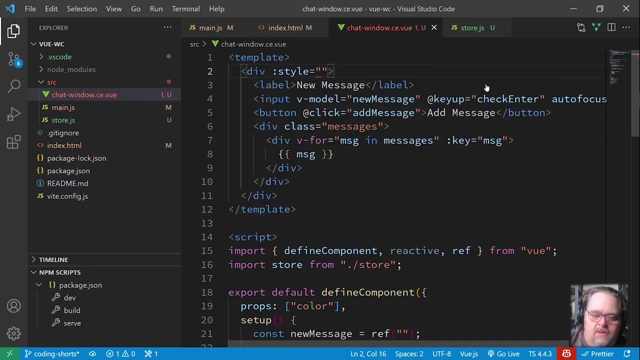 as people type: just say: go ahead and create this element here and you'll get that thing you want. and in that same idea, we come over to our view here. i'm just going to change this to be, let's just say, color. so we'll go ahead and bind to style equals color on color. if it likes that, okay. 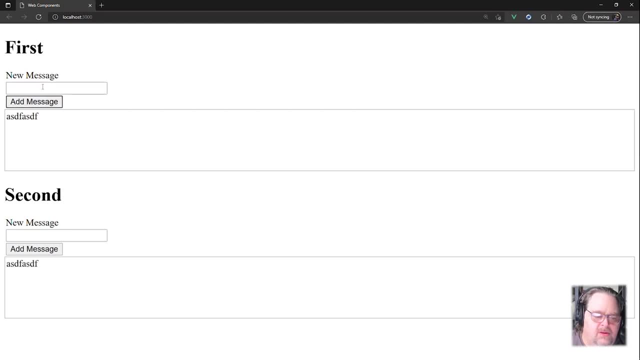 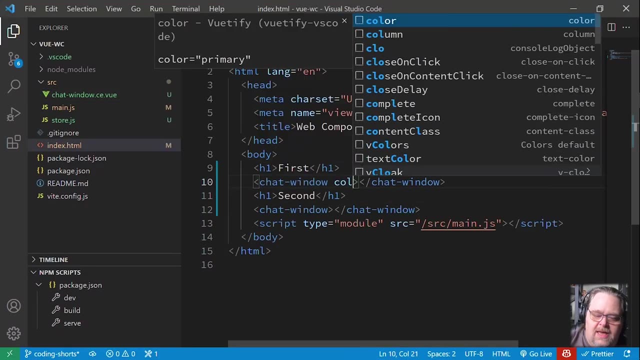 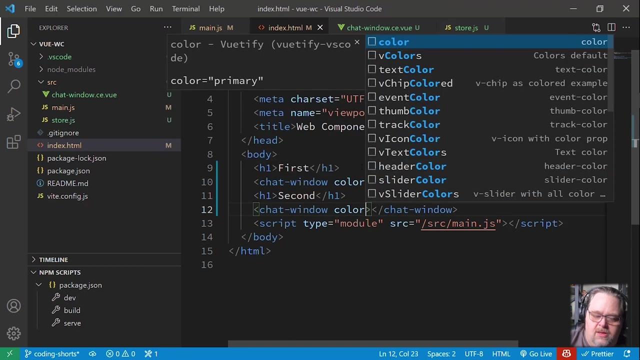 and we can see nothing's really changed. here we have the same. but if we go over to index, let's add that attribute. here let's say purple, and here we'll say color equals and let's say just gray. right here we can see we're getting. 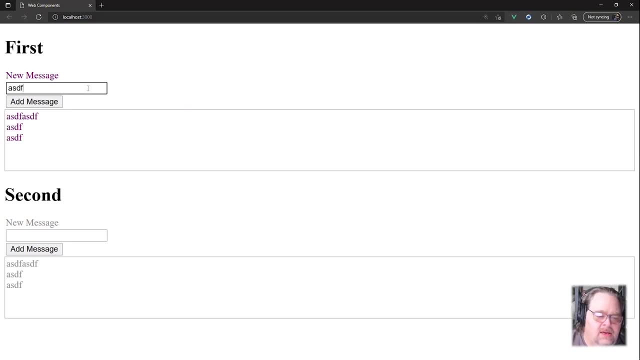 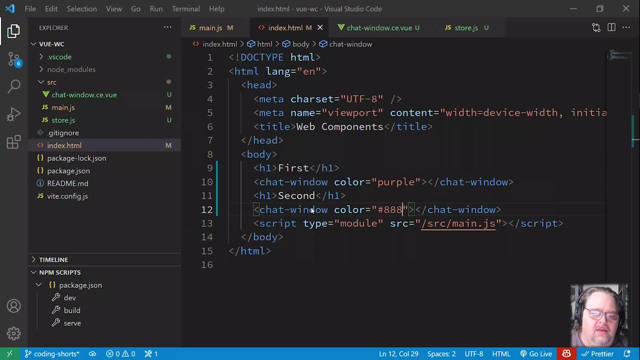 that purple and gray assigning there and even the text in there. obviously this isn't going to necessarily going to affect both, but in this way we can pass arguments back and though i'm not going to do it in this demo, we can do it in the other way. so we're going to do it in the other way.